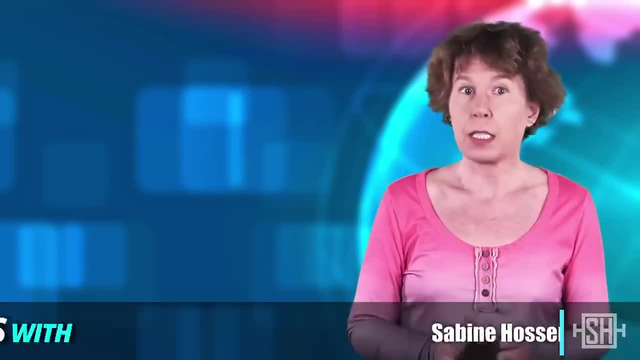 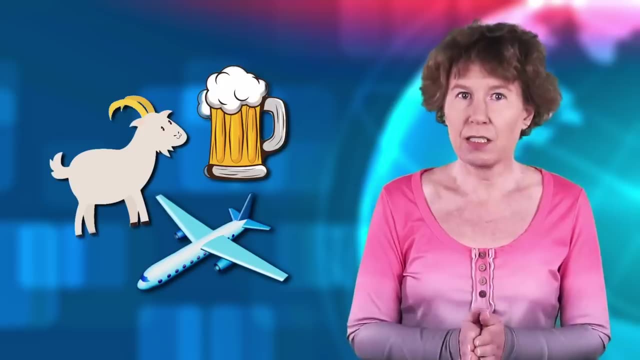 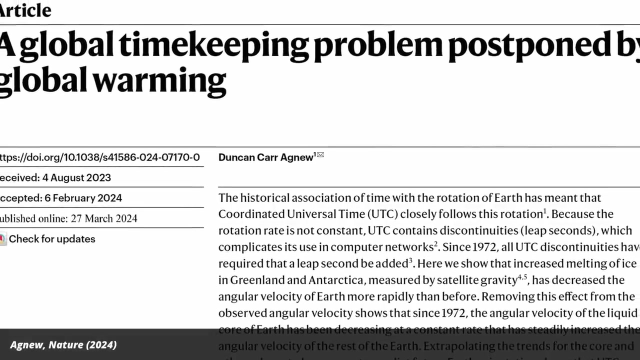 Climate change has a lot of weird consequences. It's supposedly ruining the taste of beer, makes goats shrink and flights bumpier, But I didn't see this one coming. It's making the days longer. Let's have a look. Yes, so this new study which just appeared in Nature 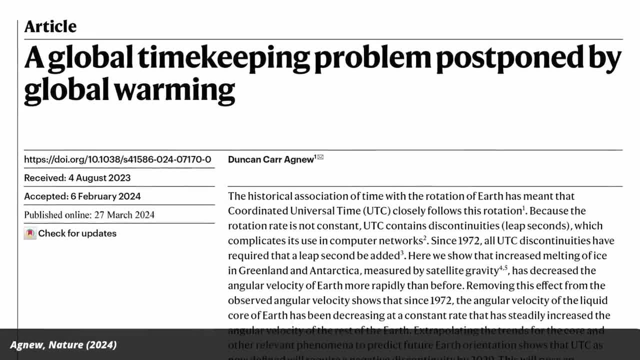 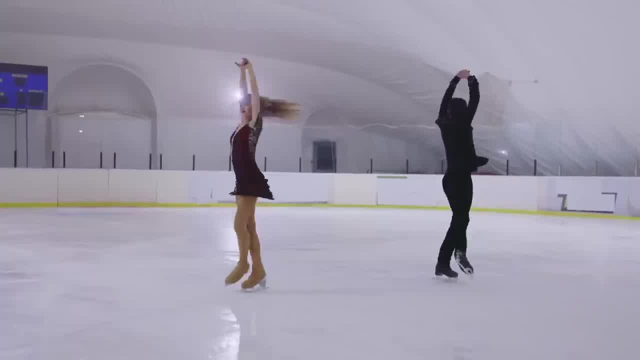 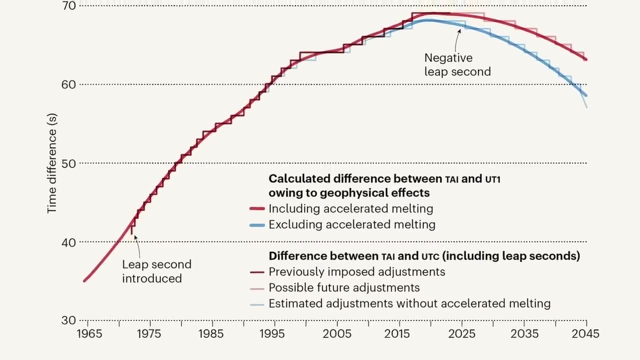 says that the melting of ice on the poles redistributes so much mass towards the equator that the rotation of earth is noticeably slowing down. It's like the famous ice dancer stretching out her arms to slow down her spin. Because of this, the next leap second to adjust for. 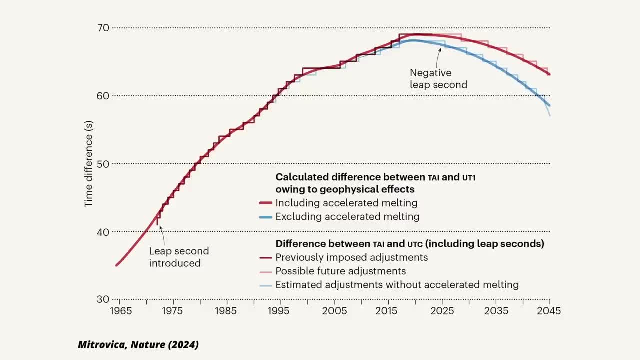 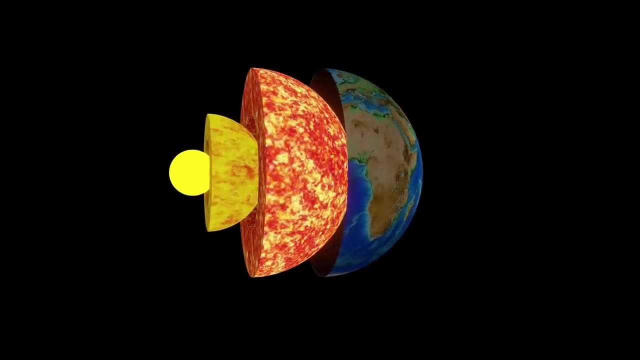 the somewhat irregular rotation of earth will have to come three years later than the original prediction said. It'll also be the first ever negative leap. second, The author says that if one takes this effect of the mass distribution from the poles melting into account, one can also conclude that the rotation of the core of earth has slowed more than previously. 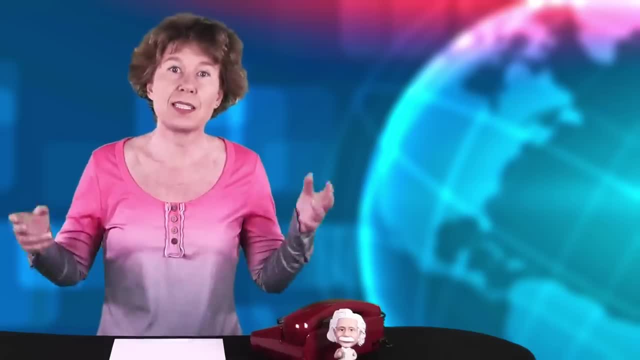 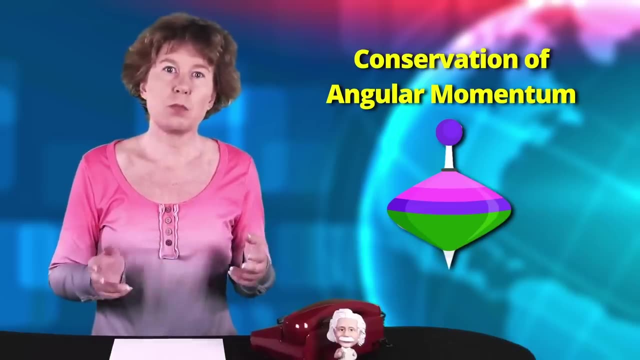 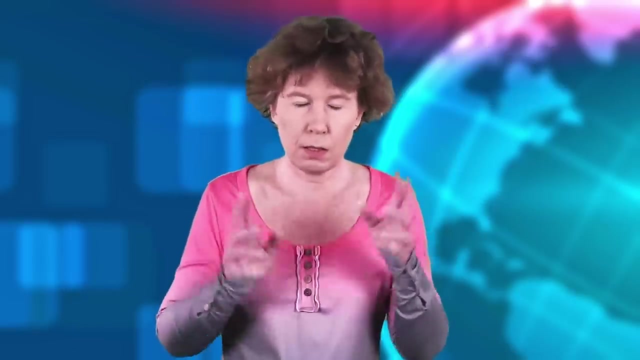 estimated. This is because angular momentum of the entire system is conserved. The more the core slows down, the more the solid crust speeds up, But the distribution of the ice also slows it down, so the core must have sped it up more. I hope I got this right. My head is spinning. 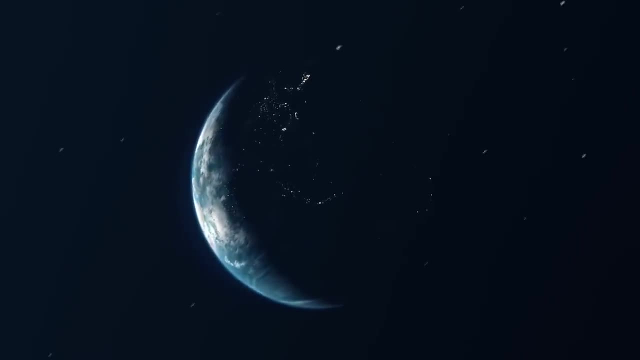 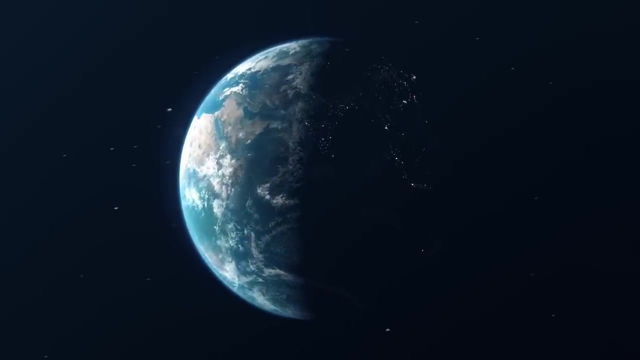 I find this completely fascinating, because you really didn't think we little humans could actually affect the spin of earth, woohoo. But actually this isn't the first time we've done something like that. A study which appeared last year found that we've also changed the tilt. 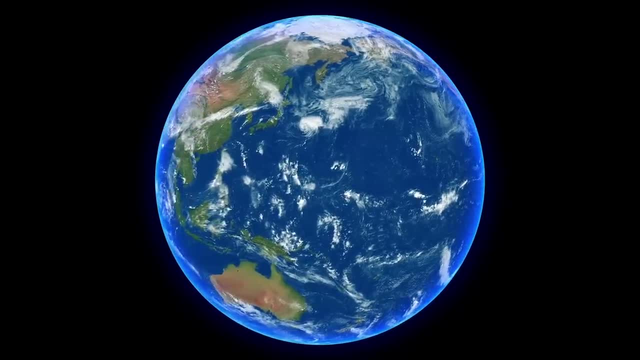 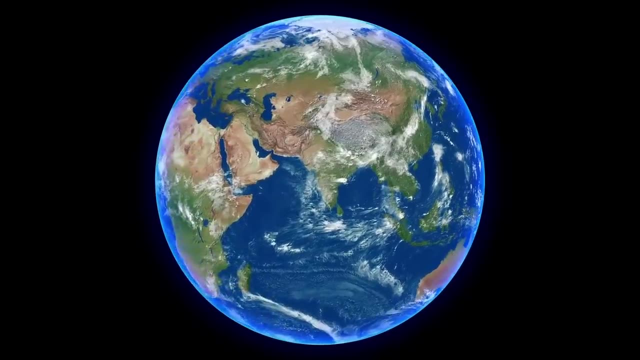 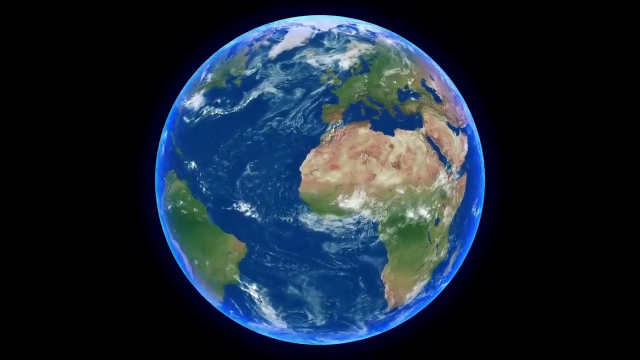 of earth's axis. The scientists figured this out by carefully tracking the spots that our planet revolves around, which, I assure you, are not Kate Middleton and Elon Musk, but rather two places on the north and south ends of our planet, called the rotational poles Over the past, 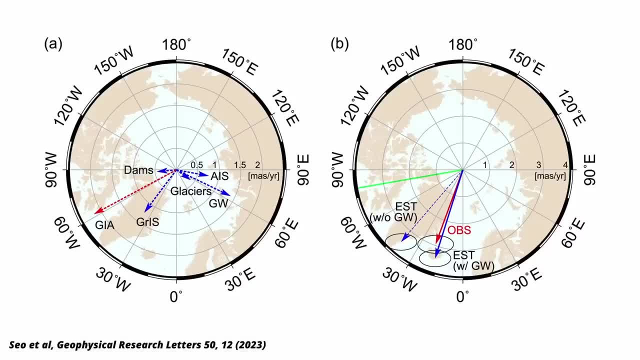 over the past 100 years, the earth's rotational pole has slowly but consistently moved westwards along this green line every year, But this changed three decades ago, when that drift began to slow and head eastward, ending up along the red line labeled OBS. The authors say that that's our doing. 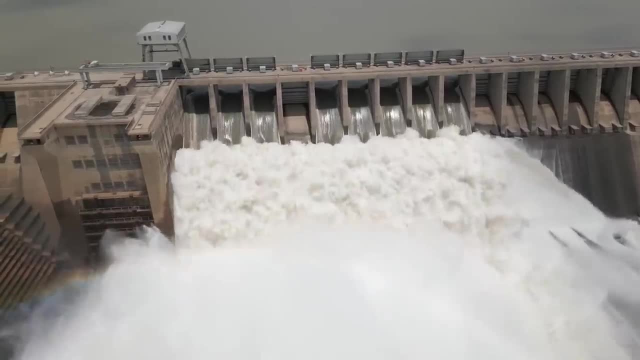 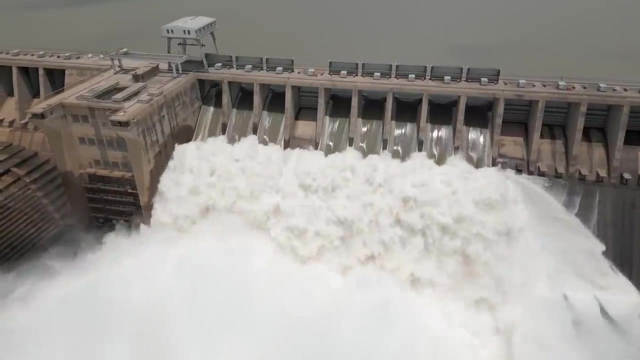 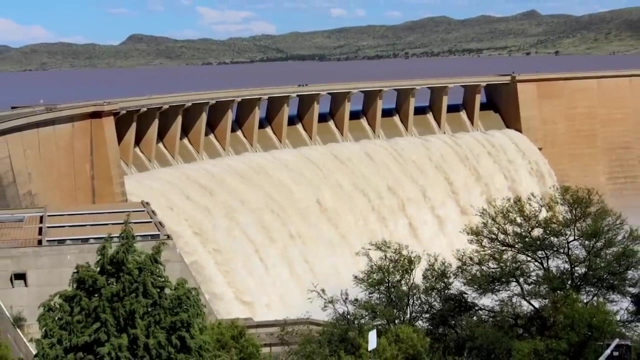 It's happened because we've pumped massive amounts of water out of the ground and used them for irrigation elsewhere. between 1993 and 2010,, we have redistributed more than 2,000 gigatons of groundwater, which shifted Earth's pulse an average of 4.36 centimeters eastward per year, adding up to 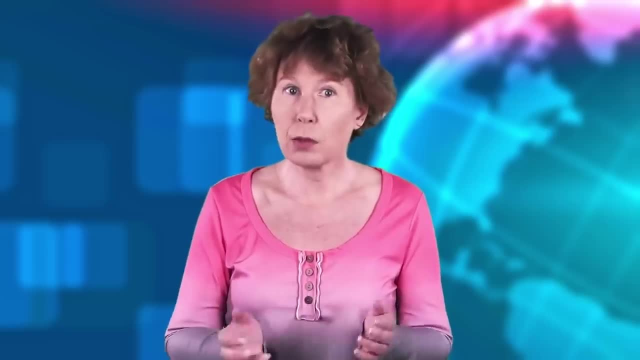 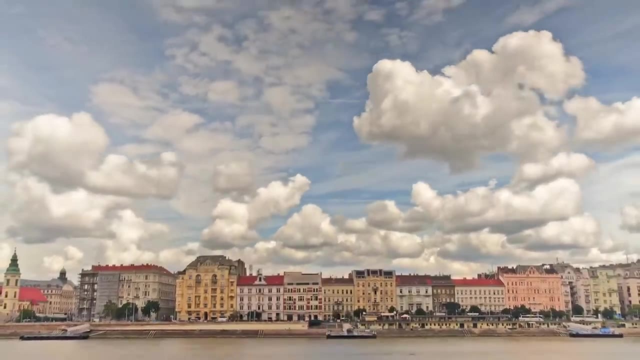 a total of 80 centimeters. The most visible consequence of this steady eastward drift is TikTok. Another peculiar consequence of climate change that doesn't get the attention it deserves is global stilling. sounds like a euphemism for the Twitter exodus, but actually. 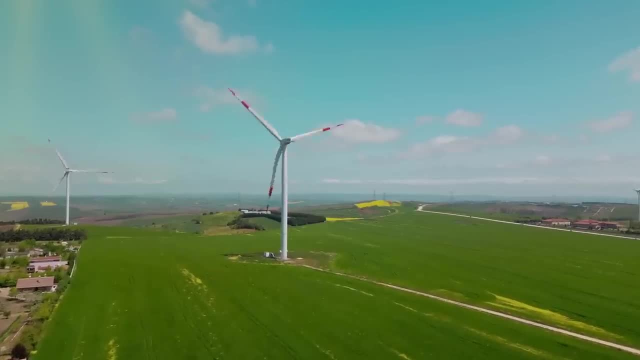 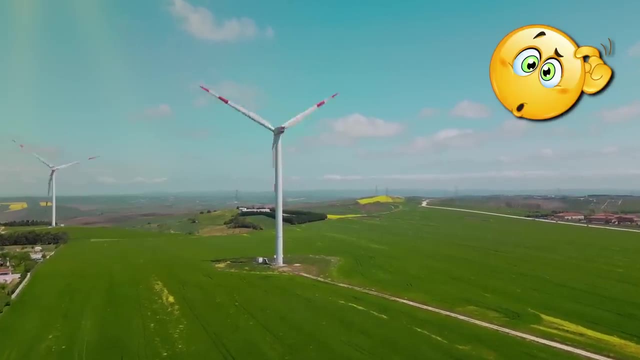 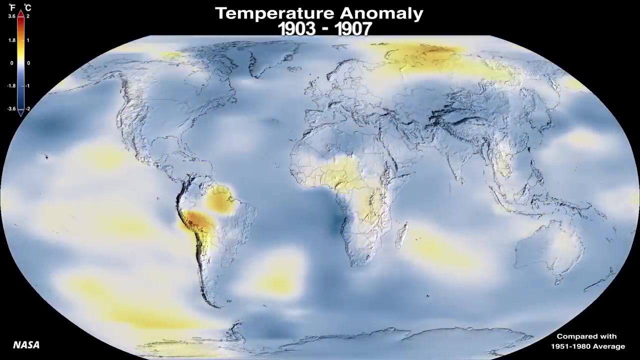 refers to the decrease of wind speeds. that might bring trouble for countries who have banked on wind power. I say might bring trouble because so far the evidence is somewhat unclear, But the general effect leading to this global stilling is reasonably well understood There. 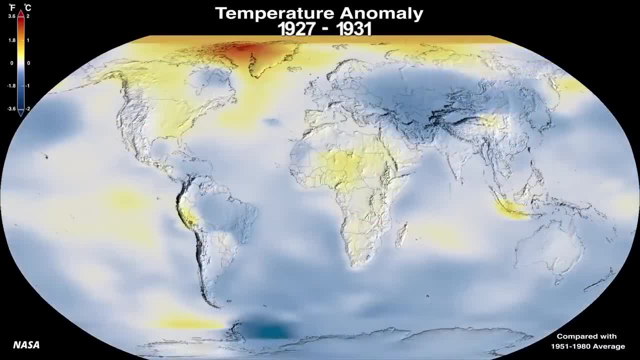 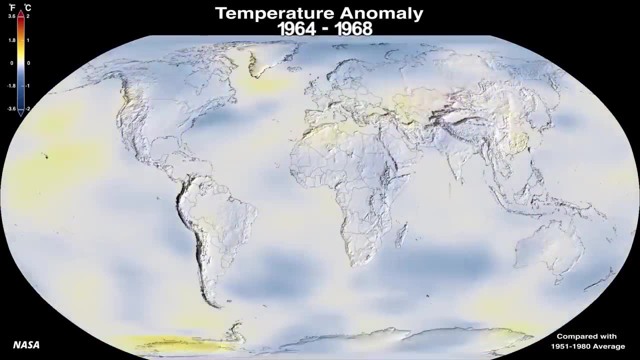 are two major causes of the wind patterns on our planet. One is the rotation of the wind, One is the rotation of the wind. One is the rotation of the wind, One is the rotation of Earth. The other is that the air is warmer near the equator and colder towards the poles. The thing is now that climate change is warming the poles faster than the equator, which decreases the temperature difference and calms down the winds. Because of this, the Intergovernmental Panel on Climate Change predicts that winds will slow down globally in the coming decades- By 2100, they say- average annual wind speeds. 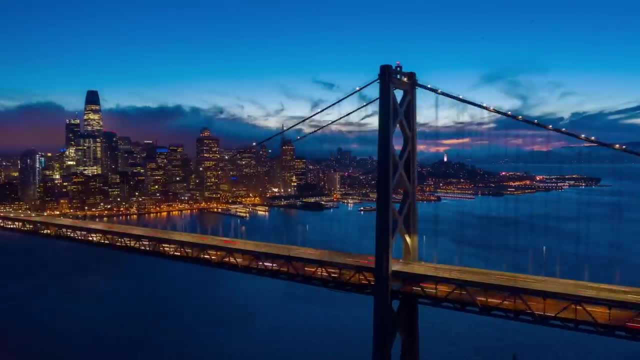 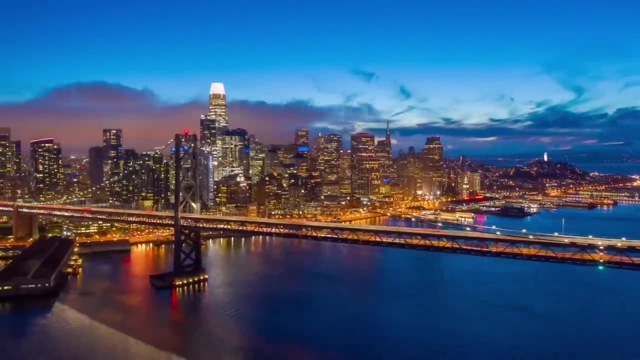 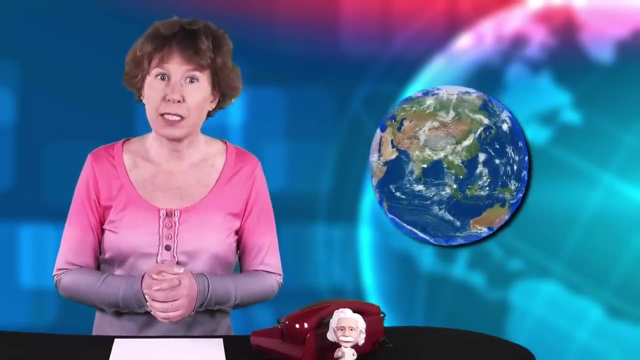 could drop by up to 20%. Climate change isn't the only contributing factor. Increases in surface roughness from cities also slow down winds. Indeed, the changes in global wind patterns could also – wait for it – affect how fast the Earth spins. It's because the angular momentum of the 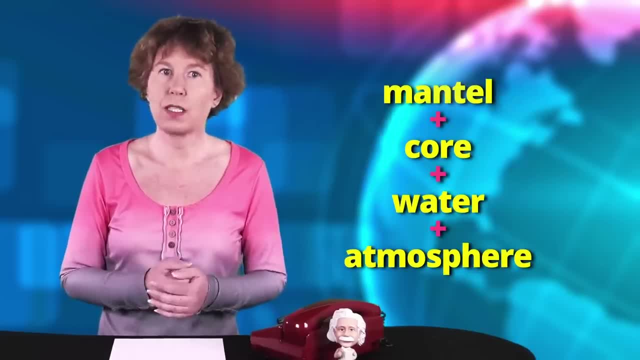 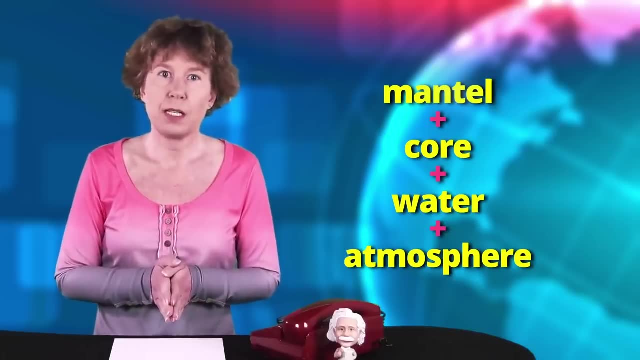 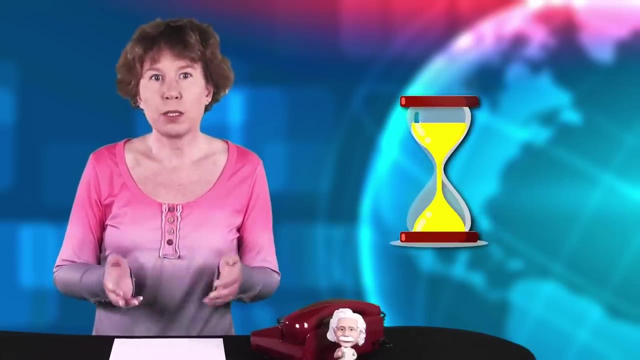 entire system, Earth's mantle called water and atmosphere, is conserved. If the atmosphere goes around less fast, then the Earth's mantle have to speed up. Now we're talking about changes of microseconds per day, so not like we'll get to sleep in forever after. But 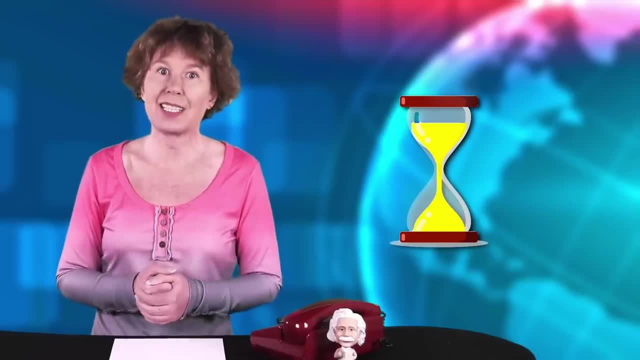 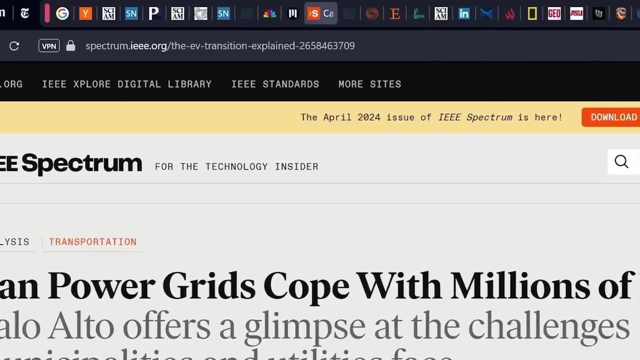 you'll get to watch a few more of those microsecond videos that are coming up any day now. I'm sure Do you know this problem that you have like a thousand browser tabs open and they get so small you can barely see them. That's why I used to have several different browser. 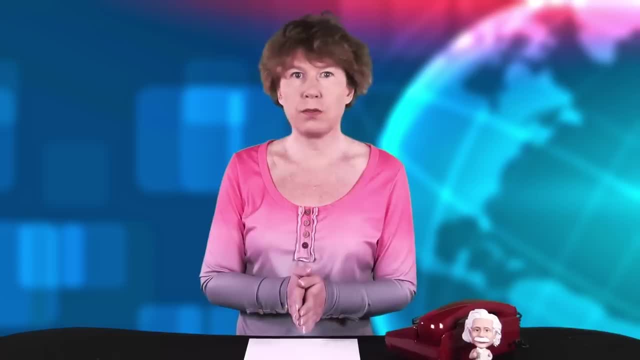 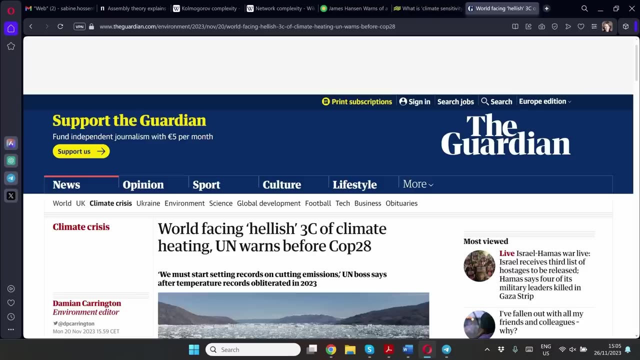 windows open and then I couldn't find the right one. Ugh, All very annoying, But I've recently switched to the app that we're using today, And it's actually a great- the Opera browser, and it's so much better. First of all, it's dramatically faster.